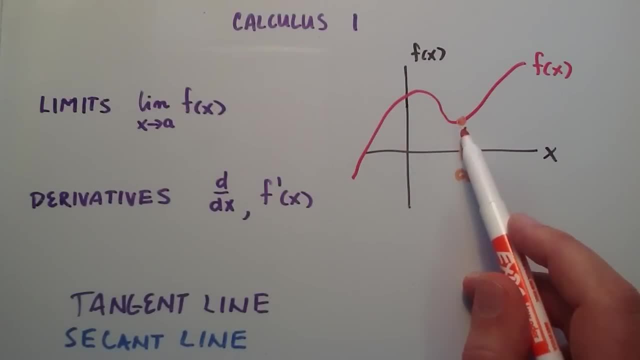 So it's like evaluating a function without actually evaluating it at that point You're evaluating it by approaching it. So the second concept is a derivative. So if we were to find the derivative of this function at the point A, basically what we're asking is: what is the slope of the function f of X at the point A? 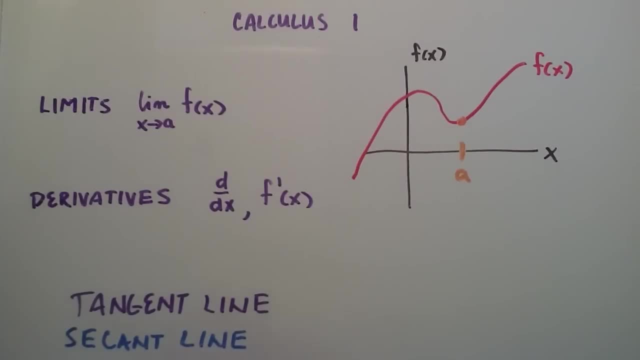 So if we were to draw a tangent line that had the same slope as our function did at that one point here, it would kind of look like this: And so if we knew what the slope of this tangent line was, then we would know what the slope of our function is. 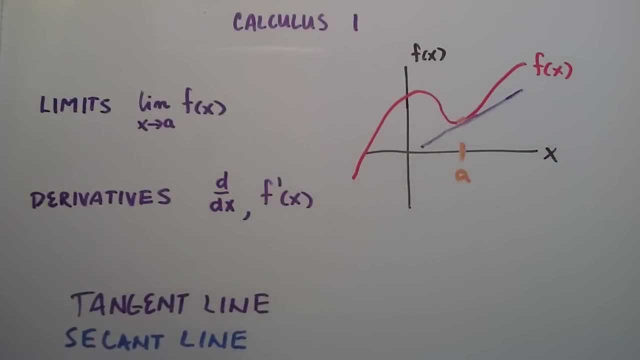 at this point. So, basically, what we're going to do is we're going to use the idea of a limit and we're going to take a secant line, and we're going to use the secant line and have it approach the tangent line. 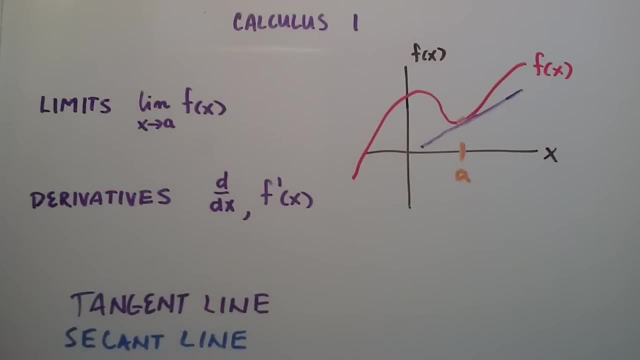 And as the secant line approaches the tangent line, then the secant line and the tangent line will have a known slope. So for example, we could kind of approximate this line With the tangent line or a secant line by having a point here and then we connect it to the point of interest here. 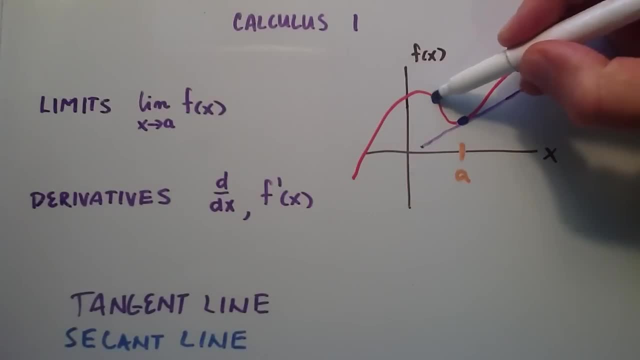 And so the reason why we want to use a secant line is because it has two points And a line that we know two points of we can calculate the slope. So that's our first approximation. It's really bad. 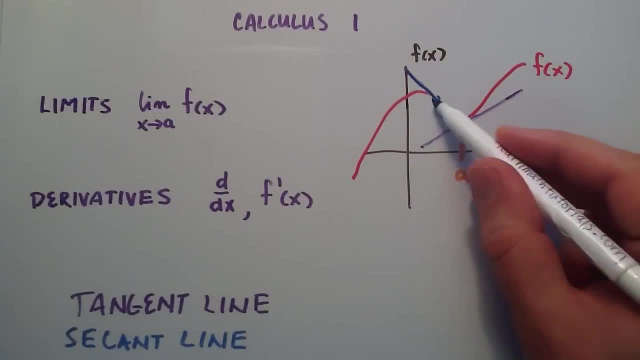 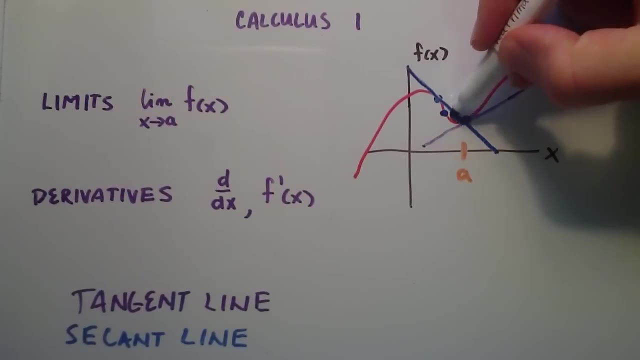 It doesn't look anything like our tangent line. But if we were to kind of move this point in on the function a little bit- let's say we put it here and then connect those two points- we could figure out what the slope of this line is. 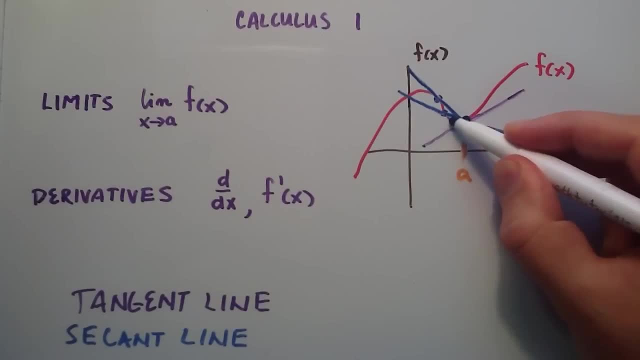 It's a little closer, but still pretty bad. We can move this in a little closer here, And now we're starting to. if we connect those two lines, we can find the slope of this line. now We're starting to get closer to the slope of our tangent line here.